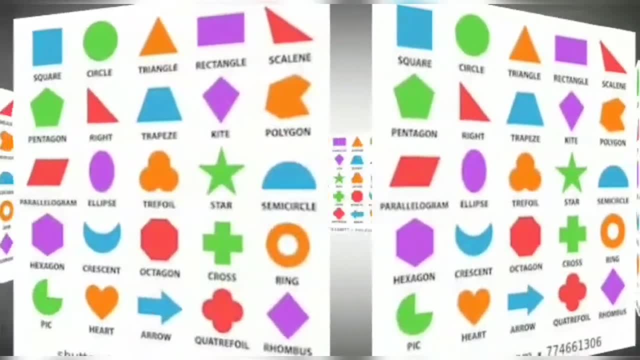 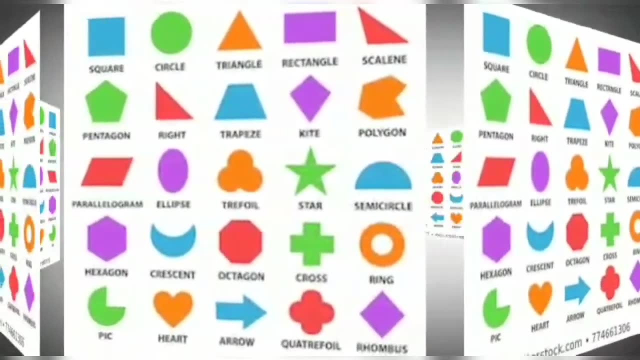 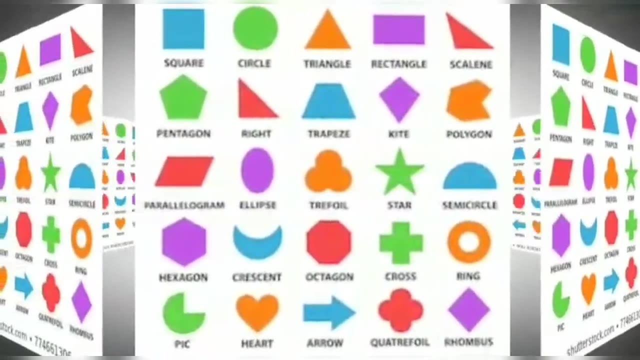 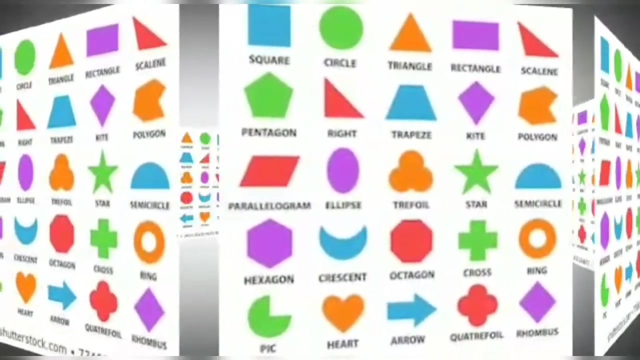 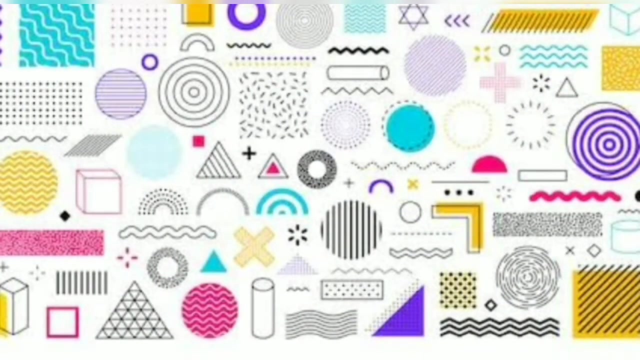 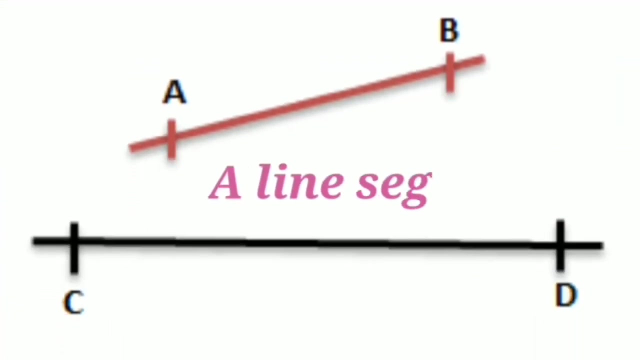 edges, planes and circles. in our surroundings We can see corners, edges, planes and circles. measure line segments. In the earlier chapters we have already studied about the line segment. A line segment is a fixed portion of a line, hence it is possible to measure The measure of each. 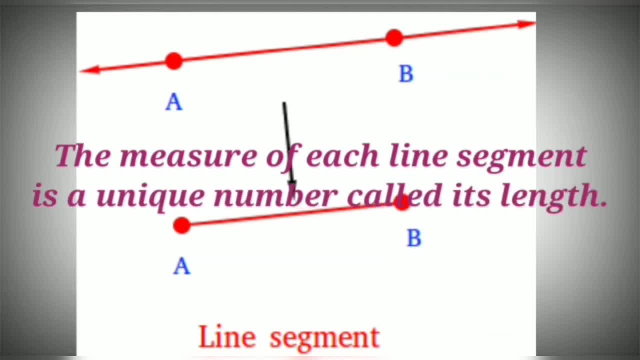 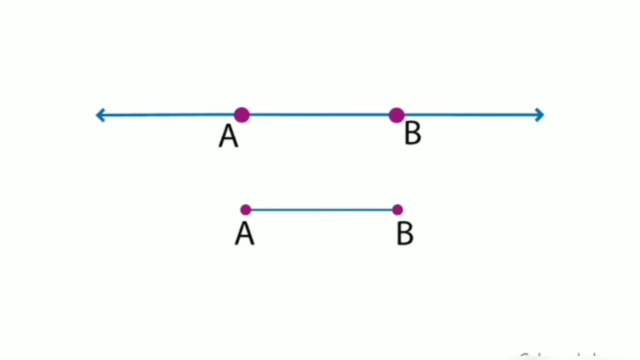 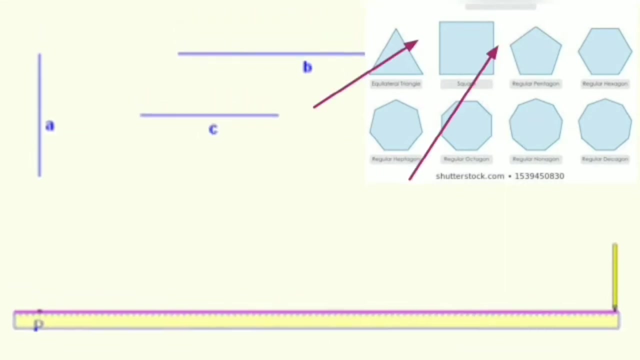 line segment is a unique number called its length. Using this idea, we can compare line segments. We have different methods for comparing line segments. This is used to refer to the various line segments. we can gather We all know about how line segments appear from different line segments. 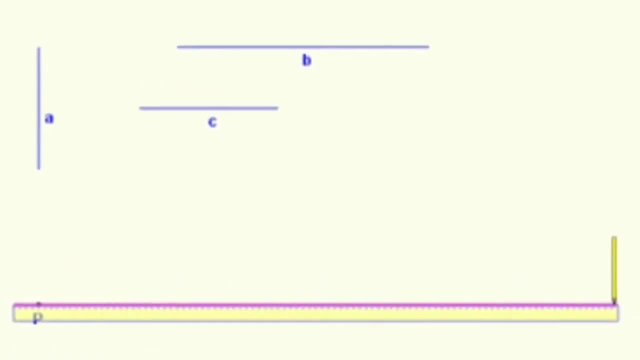 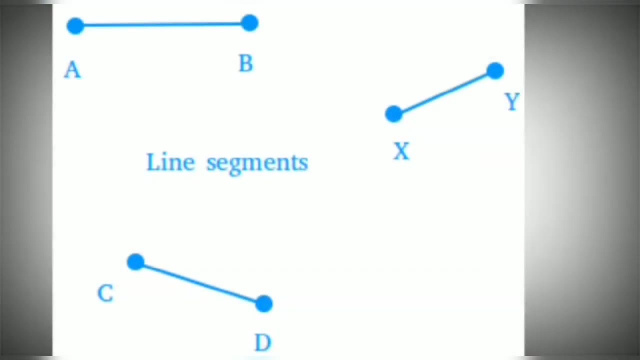 Line segmentool is anti-directional and fixed ALOT. The ratio of the two lines is one number and we call it as the ratio of the two lines. We use this information to calculate the different lines. To calculate any two lines, we find the relation of the two lines. 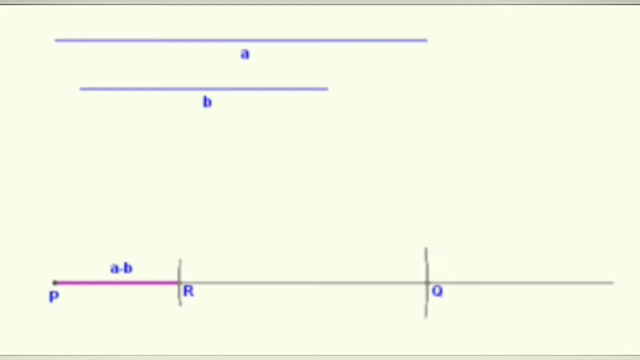 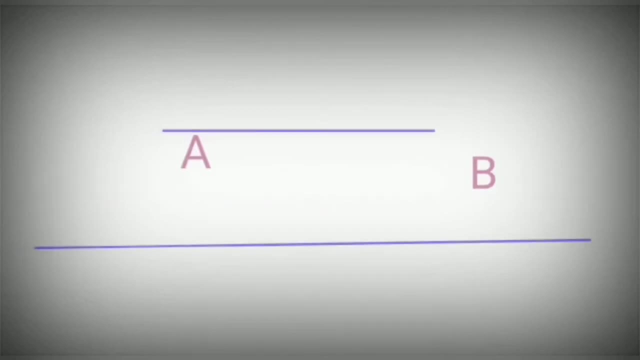 We do this in a simple way: Comparison by observation. We can compare line segments simply by looking at them. For example, here AB and PQ. Here PQ is greater than AB. Sometimes we cannot be sure about the measurement. For example, in these lines we cannot be sure. 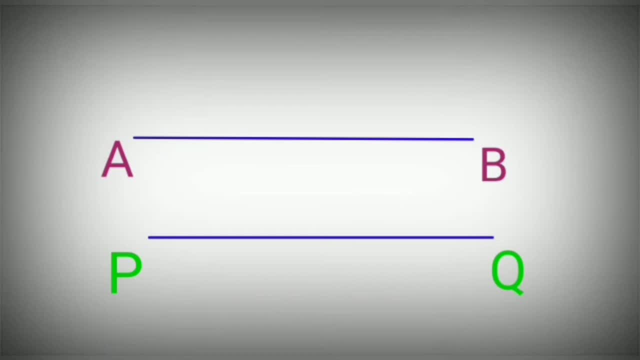 which line segment is greater than the other simply by looking at them. So we cannot rely on this method for accurate measurement of line segments. Now let us look at the whole from the perspective of observation. It is not possible to say which line segments are there from the perspective of observation. 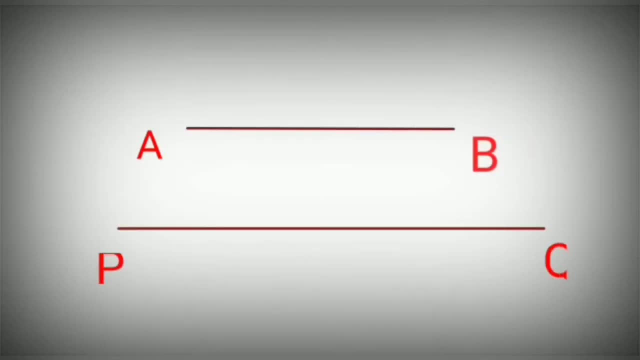 Here AB and CD or PQ is greater than the other. Here the line segments of PQ are the same, So we can say that PQ is greater than the other as well. In this picture we can see the line segments of PQ. 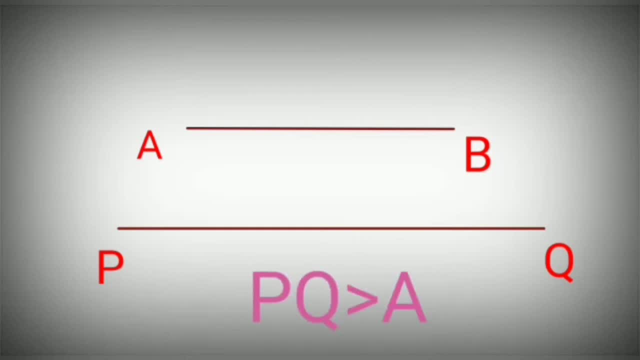 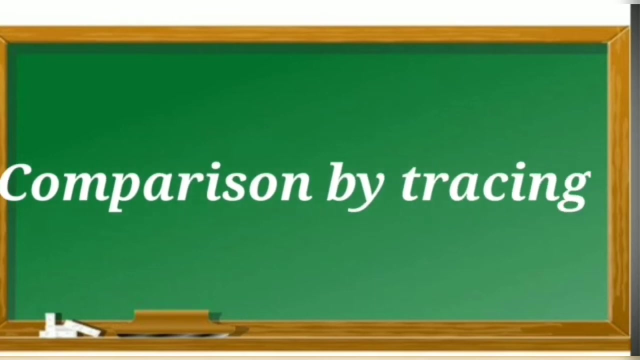 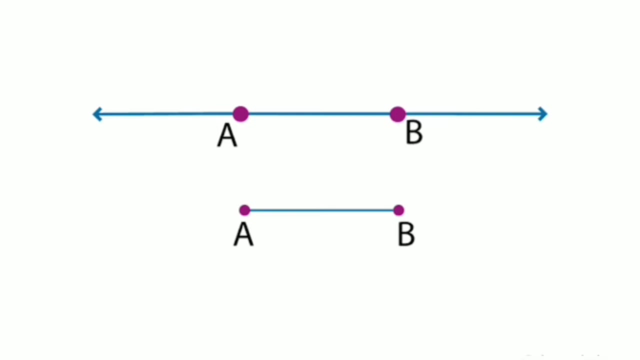 PQ is greater than AB. Here PQ is greater than AB. So we can say that PQ is greater than AB. Here PQ is greater than AB. comparison by tracing. another method of comparing line segment is by tracing using a tracing paper. trace a, b and place it on cd. now we easily tell that cd is greater than a- b. the method depends. 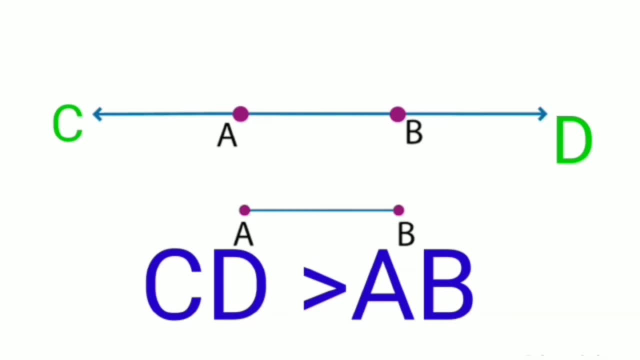 upon the accuracy in tracing the line segment. moreover, if we want to compare with another length, we have to trace another line segment. this is difficult and we cannot trace the lengths every time we want to compare. however, if we try to trace line segment using a tracing paper, trace handle feels more suitable. 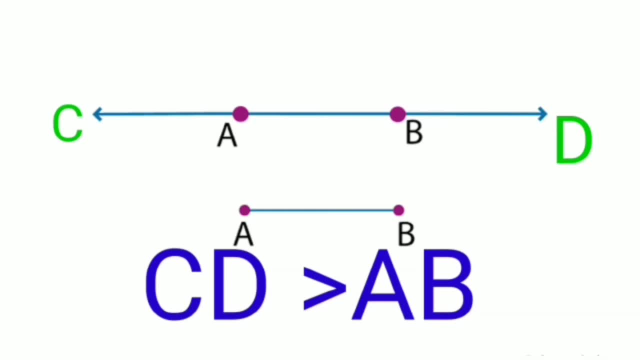 if we want to compare here also, it is likely to place a b on a b. so by this method of replacing a b with cd, it can be more successful in this action. after creating a line segment by tracing, we should follow this method of choosing a line segment. 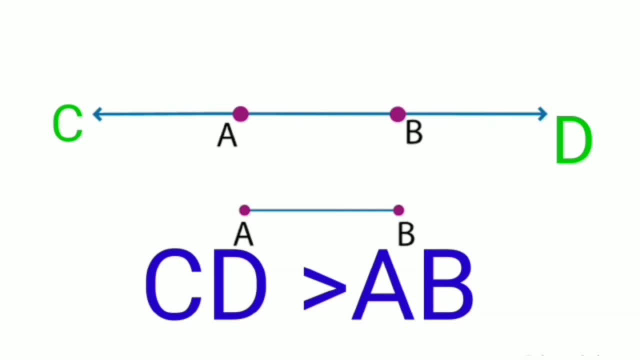 suit soother a melee. a Willam beta get a team. I thought you knew when the Rekha Canada with the one a in under and the key holy, so the key in under a car condo in a trace model a become. he do so much. see. I get a them at a with the. 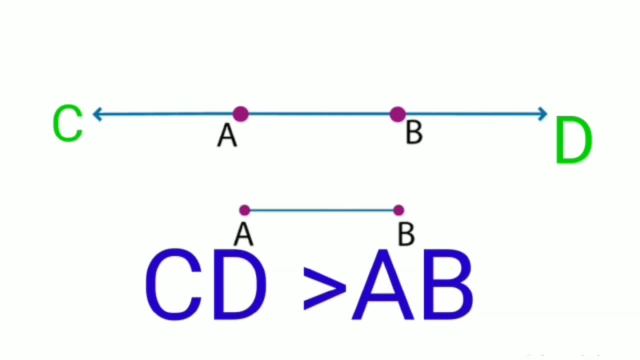 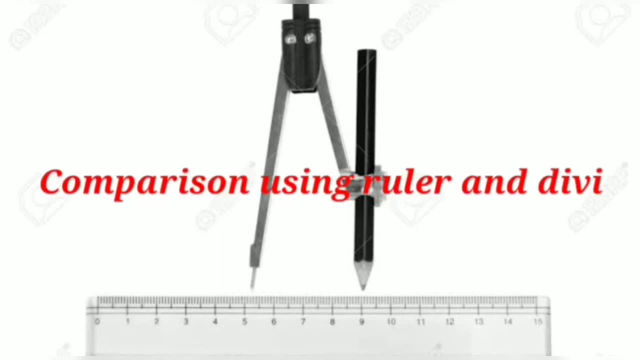 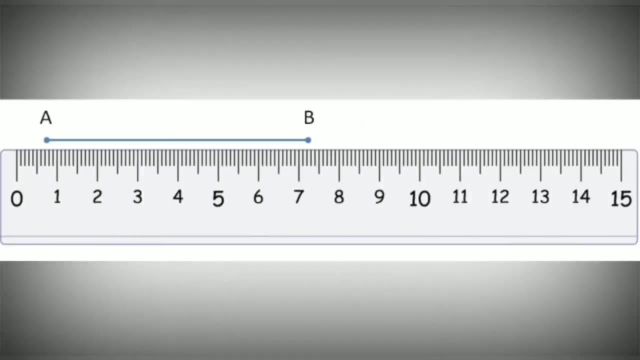 Grana, holy so Agha, pretty body trace model. the case are the aqua de la comparison using ruler and a divider. first, let us know about the ruler and a divider. a ruler, or scale, is divided into fifteen parts. each of these fifteen parts is 1 centimeter. each centimeter is divided into ten sub. 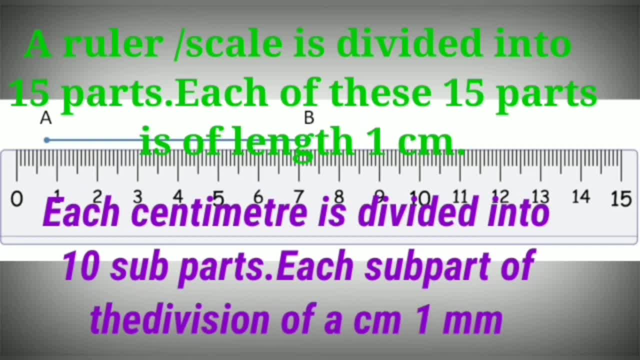 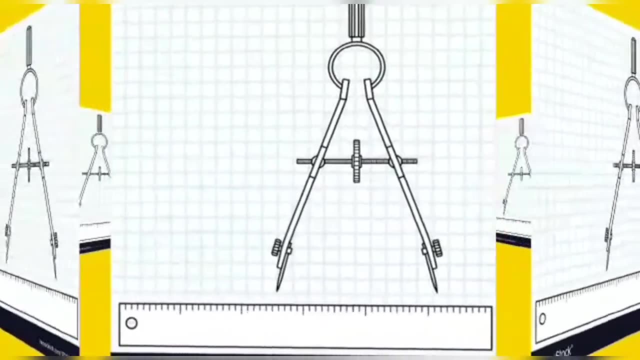 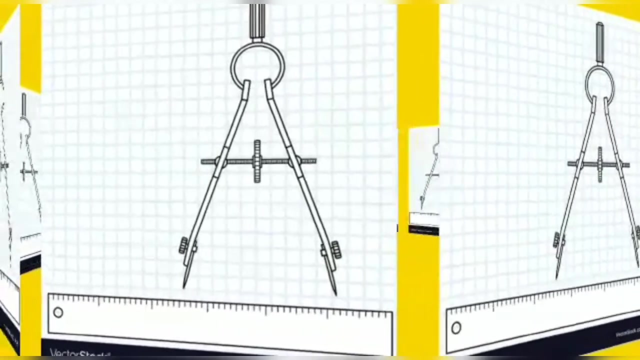 parts. each sub part of the division of a centimeter is one millimeter order, the 略" up a yogi see holy. so on the dome, Nima Salah, Karan, Agra, party gay, a petty gay at what geometry box Nellie, a lot sadhana granana, or no dirty we know. 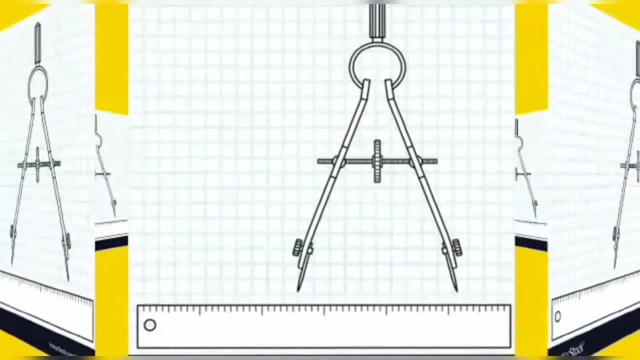 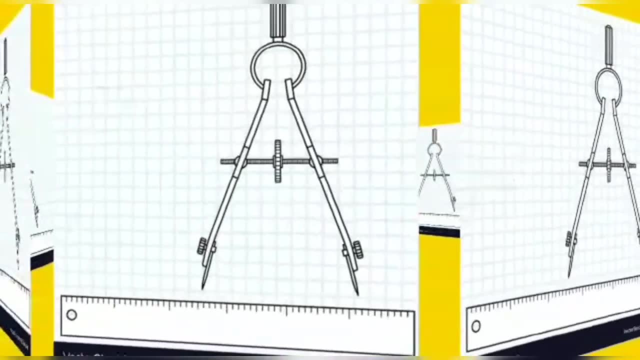 over and now. good so the case at the NAM, only the Salah Karan, Agra and again Emily are at a party. matu be positive, guru. kuda it the way I let the party a and sugar and I hate a good martyr. ah, I don't know, how did I do some of our 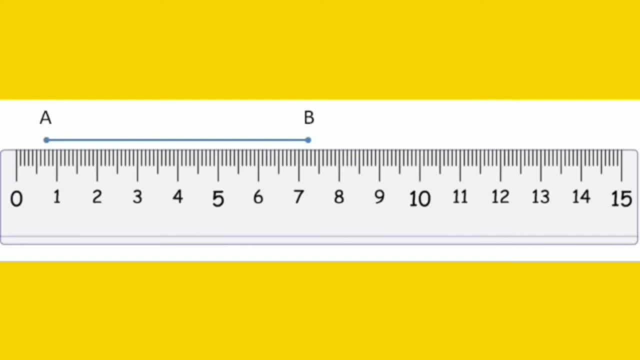 gala give it to me. he added: I do parka good Allah. one, two centimeter with the earth, a 30 centimeter and not a to be up a parka gala give a box. see pretty on the centimeter Nellie now up above ago one, two millimeter with the irritate now. 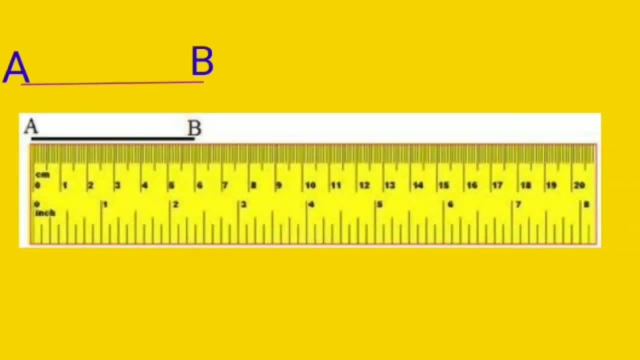 let us measure the line segment a- B. please does zero mark of the rule. let us measure the line segment a- B. please does zero mark of the rule. let us measure the line segment a- B. please does zero mark of the rule. at end of the line segment say a, read the mark against B. it is 5 centimeter so 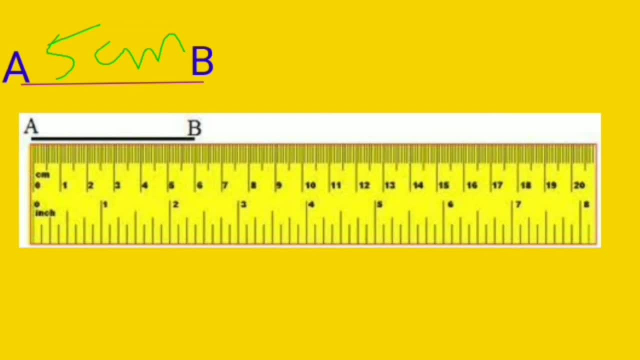 the length of a B is equal to 5 centimeter. Naviga are at the party. a sahayad in the even do a B Rekha condo anna measure. Marta got the. Marta got more. a Yasatori on a 3.0 in Sonegur 2 plausible. so we who are room out the 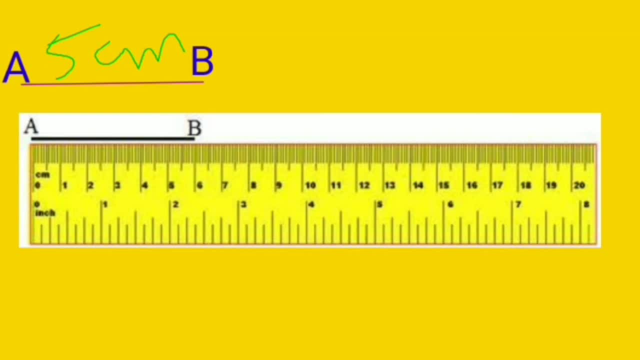 windows, Italy, optimists repeating the will S л first system name at I go to a. so the museum before the life alibi. no, there is X, the Sache contar, not us. 8th, a newfer beftari. here alibi is equal to 8 centimeter of the market. our littleuki, I do have to measure. day at the Colada their look at the whiteosity. but I am also s motive. a Nann testimonies, the dark. I'll see. see that in an interesting world. press this shape. if you look this you know we've got the color pressure. we killing LP lemon earth, that this is the. 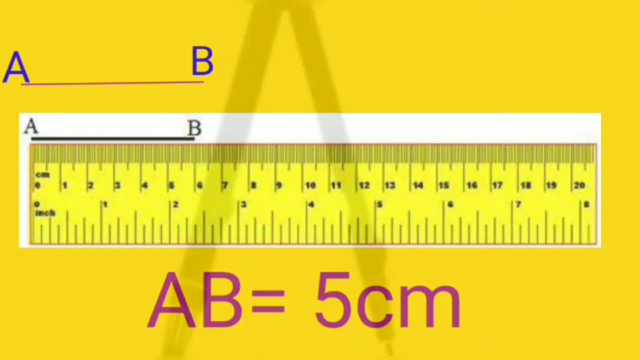 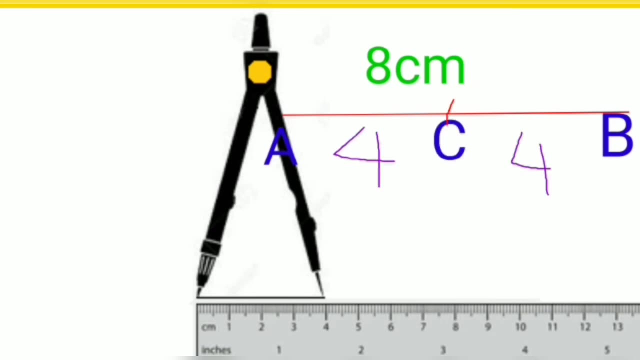 bill. we're doing it. so what does that mean? another F Epic, Rachel, that this isittle. let us draw line segment of AB of length 8 centimeter. Now let us measure AC: It is 4 centimeter. Also, BC is of length 4 centimeter. So we say that C is a midpoint of AB. 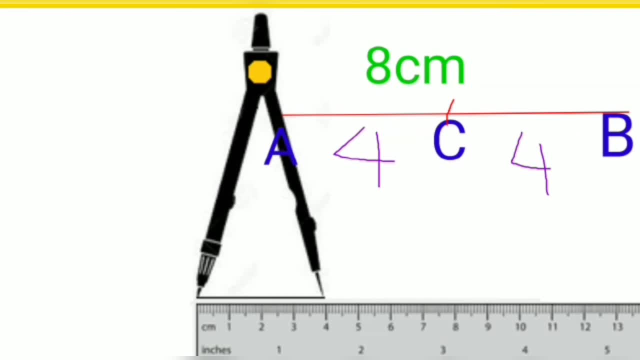 After that we have to write AB of length 8 centimeter. Also, we have to remember BC of length 4 centimeter. So now we have to write C of length, AB of length. So now we have to remember BC of length 4 centimeter. 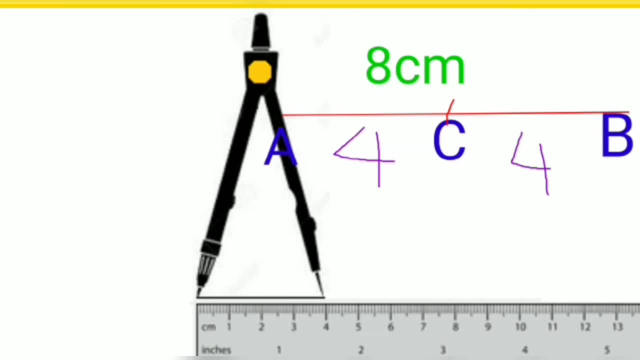 So now we have to remember BC, of length, 4 centimeter. After that, to measure a line segment by a divider open, it place the end point of one of its arms at A and the end point of the second arm at B. 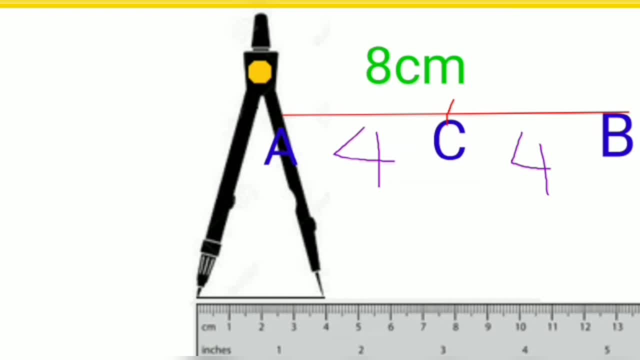 Taking care that opening of the divider is not disturbed. Lift the divider and place it on the ruler. That one end point is at the zero mark of the ruler. Now read the mark against the other end point. Now let us use this divider to measure the triangle. 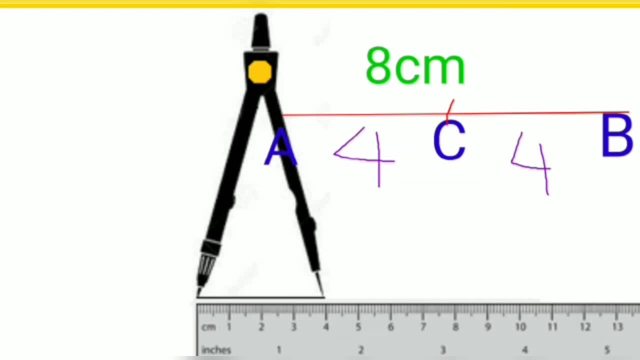 To measure the triangle we have to put one piece of the triangle over the other and take B as the other piece If we wish to derivate the triangle either. a year to DNA are at a party a melee it beck one to do the you in to.